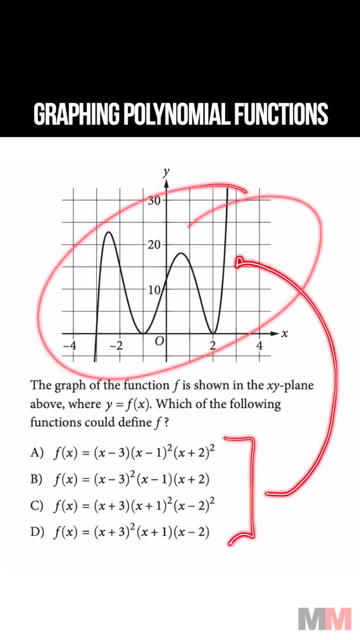 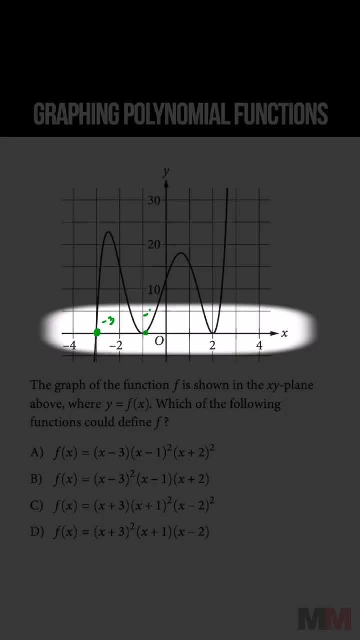 You get a graph above which one of these functions defines that graph. So the first place you're going to have to look at are your roots or your zeros, And that's going to be negative 3, negative 1, and 2.. Your roots and your zeros are the x values that make your factors 0.. And if I plug in negative, 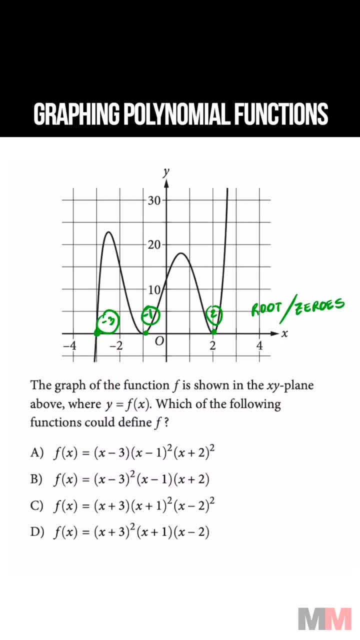 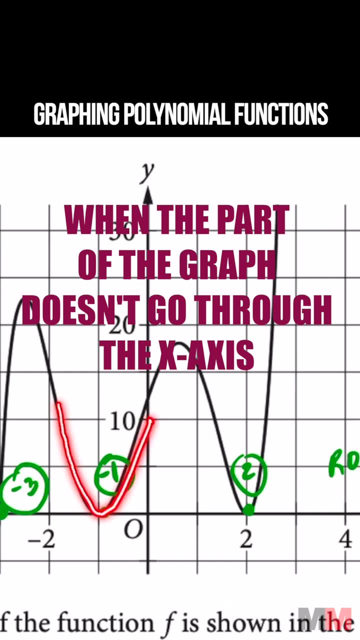 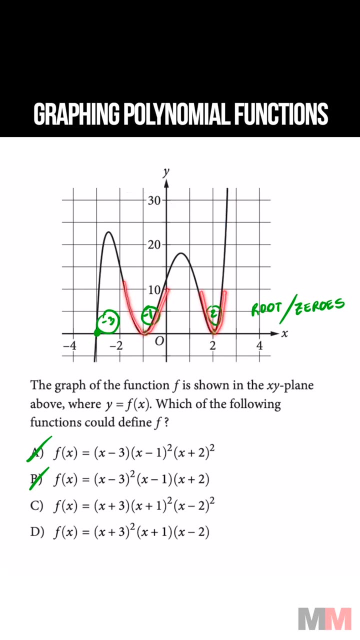 3 right here, that is not going to equal 0, meaning that a and b are wrong. When your polynomial does not go through the x-axis, like this spot right here and this spot, then that means that the factors of those roots are going to have an even exponent. Here's an easy way to remember That. 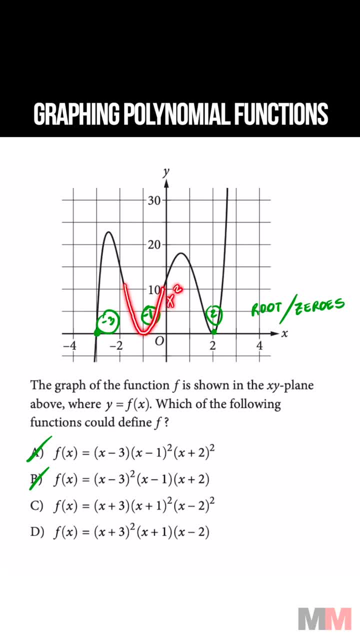 looks like the x squared function, which is even, and it does not go through. When it does go through the graph like this one, then the exponent of that factor will be odd. So that's odd, even and even, which is going to match letter choice C Peace. 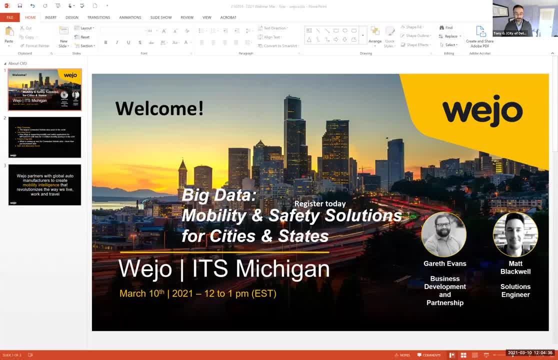 And I just want to welcome everyone to our March event of our 2021 webinar series for ITS Michigan. Today we have Weejo with us and we're presenting on big data specifically focusing on mobility and safety solutions for cities and states. And Weejo we've worked. 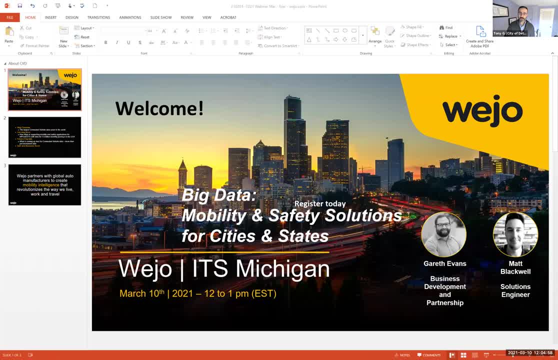 with them on a couple of potential opportunities in the past and I felt like that this specific topic is of extreme interest to our ITS members and other members here within the community. Thank you for your patience and thank you for actually joining on such short notice. 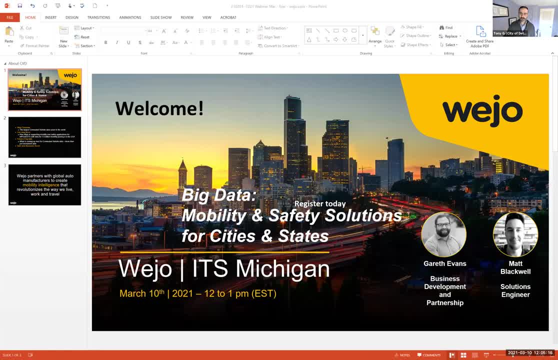 We've had a few delays and I got vaccinated on Monday, so that kind of also threw a small wrench in the wheel. But with that said, I do want to remind everyone that today's webinar is being recorded. We will be posting it on our YouTube site, so we have an official YouTube.